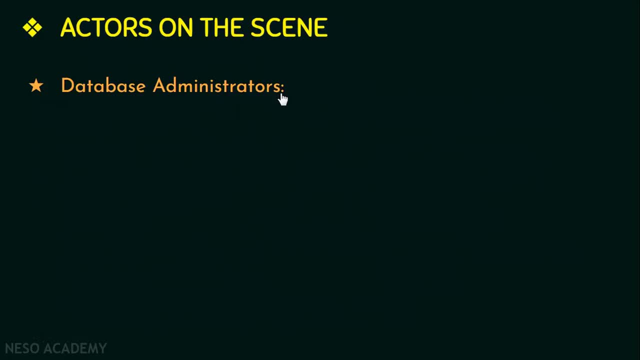 person or a chief person or a manager to manage these resources. Similarly, in the database environment we have database as the primary resource and database management system, that is, DBMS and its related software, as a secondary resource, And it is the responsibility of a database administrator or a DBA to administer the database. 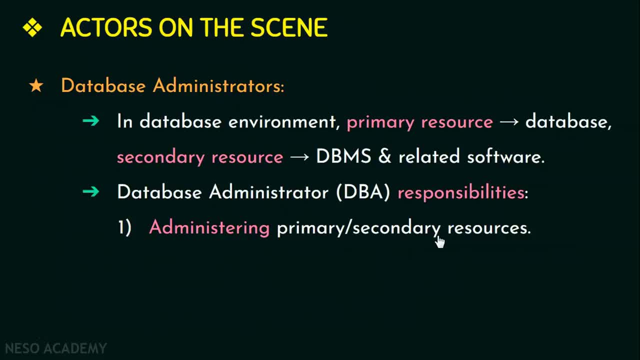 or to manage these resources, that is, the primary and the secondary resources. The other responsibilities of a database administrator or a DBA are they authorize access to the database, That is, they can grant any user the permission to access the database. And the next responsibility of a DBA is coordinating and monitoring the use of database. 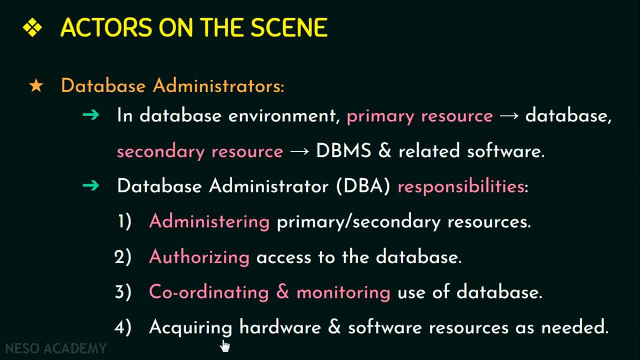 Also, a DBA is responsible for acquiring or obtaining any hardware and software that is available in the database as needed. So these are the main responsibilities of a database administrator. The other responsibilities would be troubleshooting if any problem arises or to see if there are. 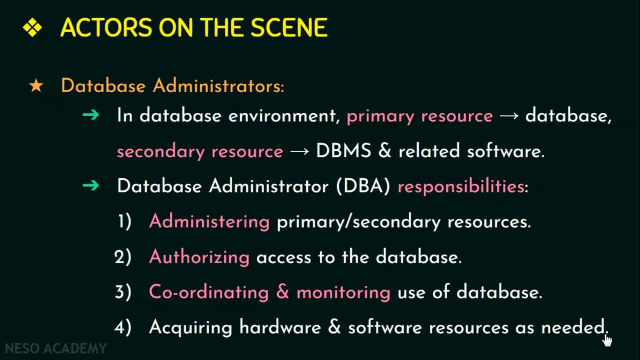 any security issues and so on. In a large organization, a DBA or a database administrator will have a support staff behind to help him with his duties and responsibilities. So that's about database administrators or a DBA and his responsibilities. Moving on to the next type of database users, under actors on the scene, we have database. 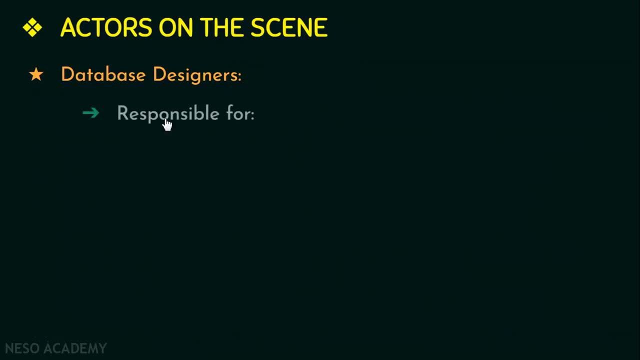 designers. Database designers are responsible for identifying the data that we are going to store in the database And, based on this data that we are going to store in the database, a database designer should choose appropriate structures to represent and store this data, And a database designer is also responsible for communicating with the database. 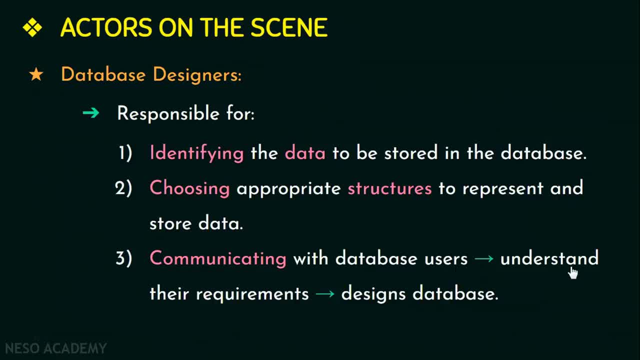 A database designer is responsible for communicating with the database users and try to understand what their requirements are And, based on their requirements, a database designer designs a database. Now, these database designers: they interact with each group of users and develop views for each of these group of users based on their requirement. 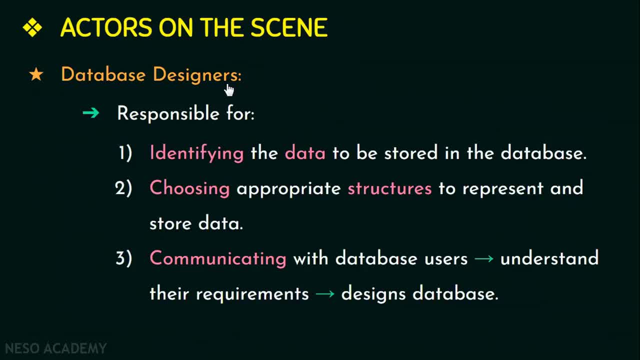 We have already seen what a view is in the previous video. A view is a subset of the database. It is derived from the main database and it only contains data that is required by a particular user. So database designers develop views for each group of users and then each view is linked. 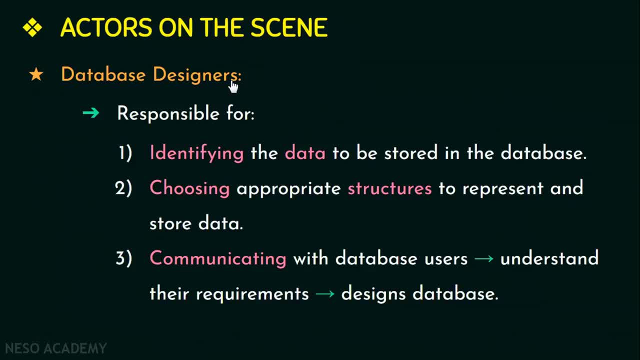 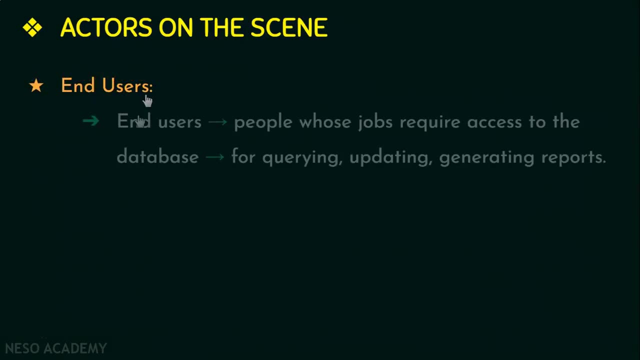 with the views of other group of users and that final database design should fulfill the requirements of all the user groups. And that is about database designers and his responsibilities. Now let's look on to the next type of database user: the end users. End users are the people whose jobs require access to the database for querying the database. 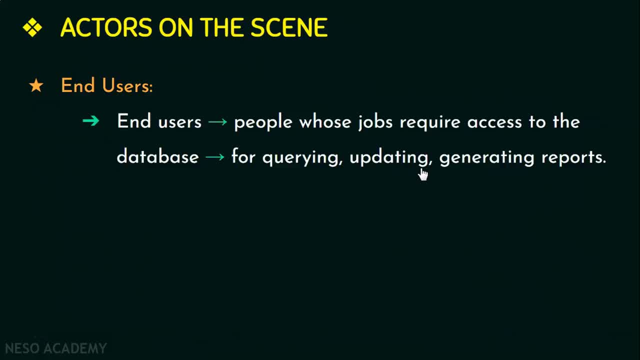 to get any data that they want or to update the database, to bring in some changes and for generating reports. Now let's look into the categories of end users. The first one is the casual end user. A casual end user accesses database occasionally, That is, they access the database not very frequently. 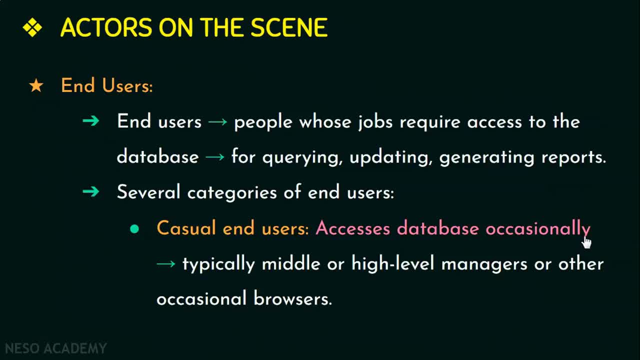 They access the database not very frequently. They access the database not very frequently, Not very regularly or not on a daily basis. They access the database only when they want to query some data or if they want to update the database or for generating reports. 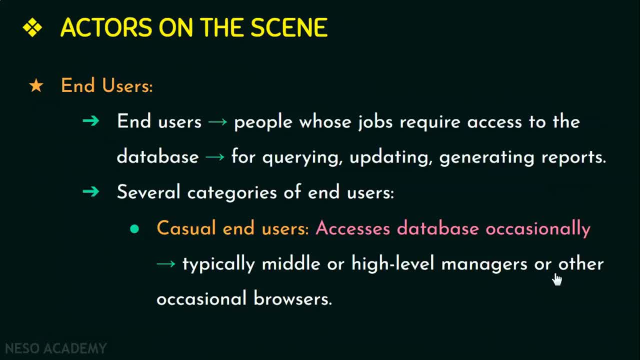 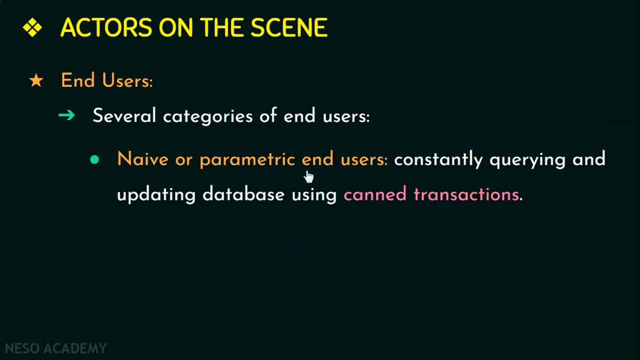 And usually the middle or high level managers or the top level managers or other occasional browsers come under this category. The next category of end users are the naive or parametric end users. Most of the end users come under this category And these end users. 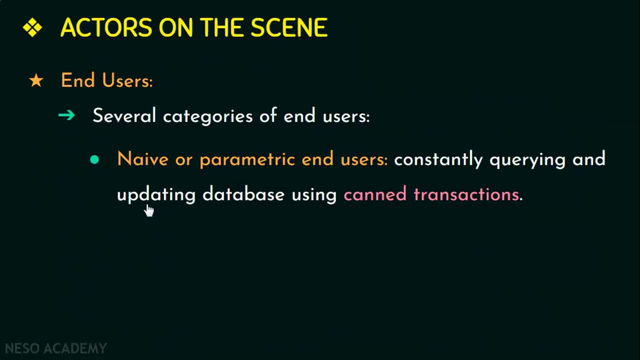 Constantly query the data from the database and also updates the database for any changes using canned transactions. Now, what are canned transactions? They are the standard type of queries and updates: to query the database for some data or to update the database for some changes. 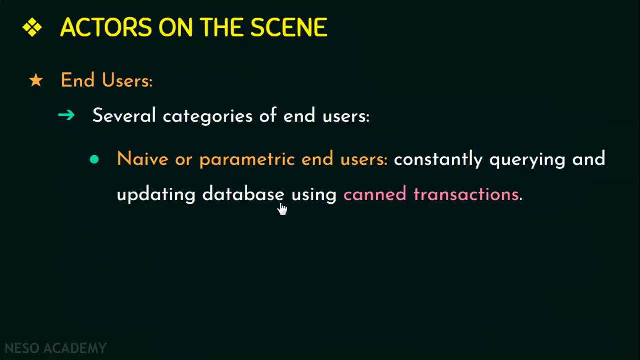 Like, for example, a reservation agent for probably airlines or hotel or train or bus, As per the request from the customer, They check the availability of the data. They check the availability of the data. They check the availability of the data And make reservations. 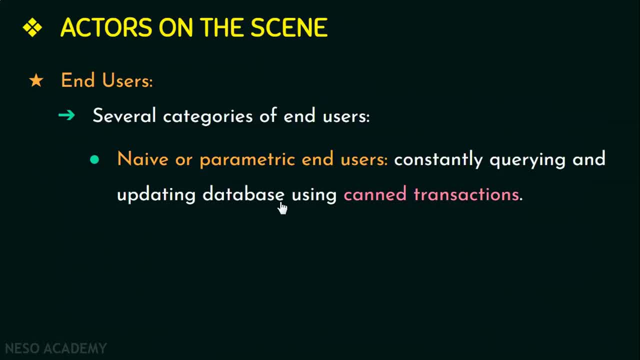 On a daily basis. they use similar set of functions to make reservations or to check for availability, And so they have a predefined set of queries or a standard type of queries to query any data that they want or for updating the database for some changes. The next category of end users are the sophisticated end users. 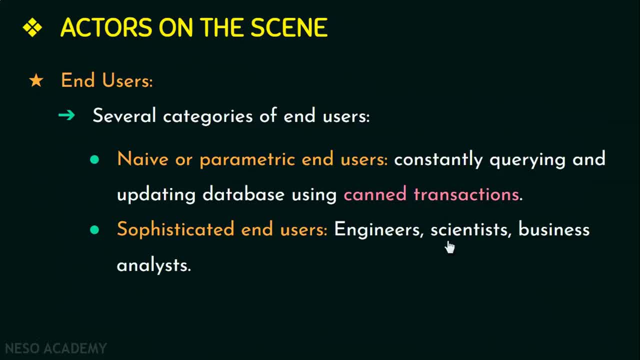 Sophisticated end users are the engineers, scientists, business analysts and any other end users who are familiar with the DBMS or the database management system and the facilities that the DBMS provides. They develop their own database applications to meet their requirements. And then we have the standalone users. 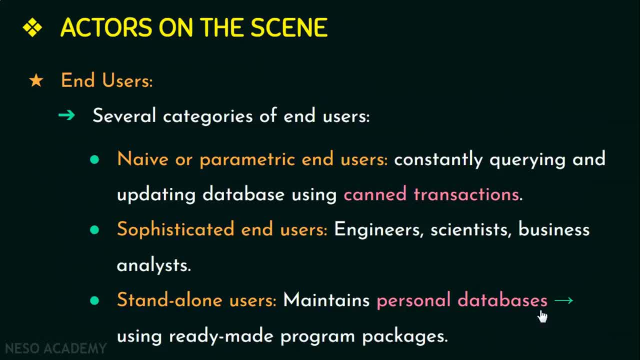 These users maintain personal databases by using ready-made program packages. Now, for example, a person running a business would like to keep track of his personal financial data for tax purposes, So for that He maintains his own personal databases using the ready-made packages, And these ready-made packages would be either menu driven or graphic based interface. 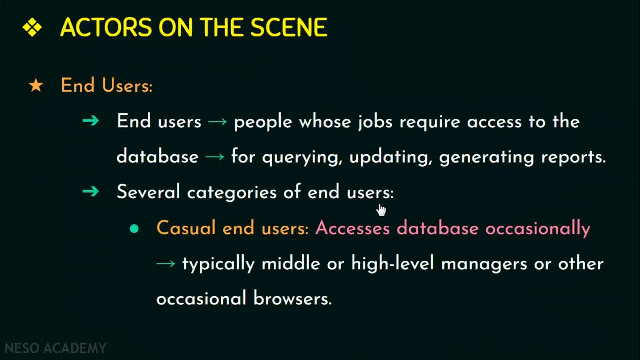 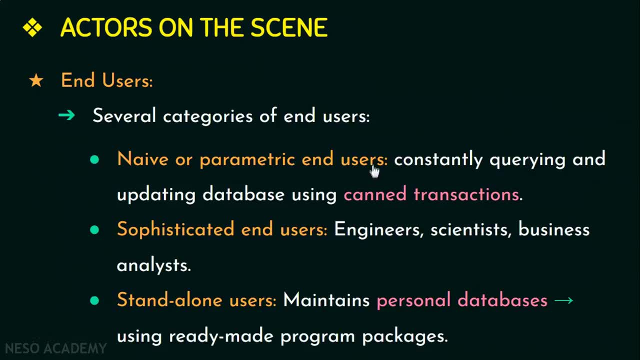 So that's all about the end users and the categories of end users. The casual end users and the naive or parametric end users don't know in detail the DBMS facilities, whereas the sophisticated end users are experts or know much about the DBMS facilities. to 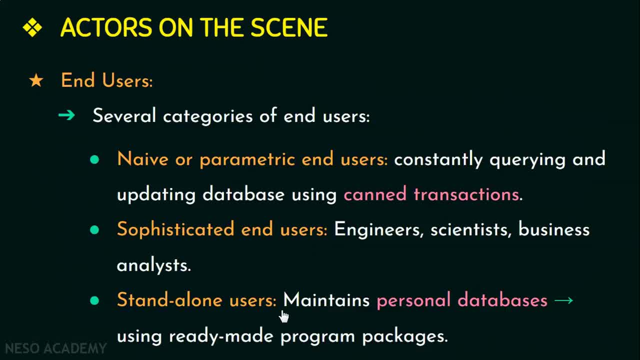 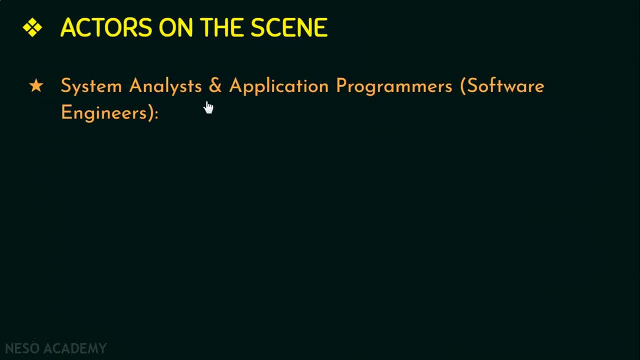 satisfy their requirements, And the standalone users are experts in the ready-made packages that they use. Now. the next type of database users are the system analysts and application programmers, or otherwise called as a software engineers. The system analysts determine the requirements of the end users, especially the naive users. 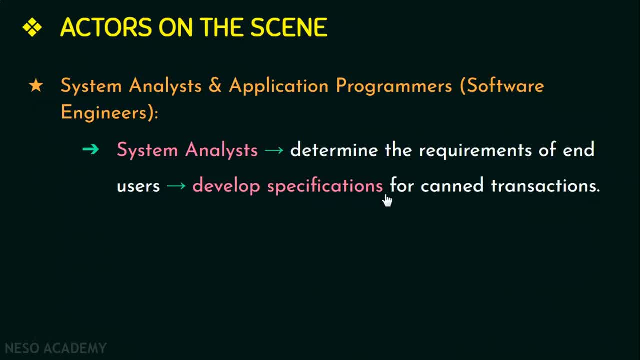 or the parametric end users and then develop specifications for canned transactions. We have already seen what a canned transaction is, So a system analyst, based on the requirements of the end users, will design these standard types of queries, And an application programmer is responsible for testing, debugging, documenting and maintaining. 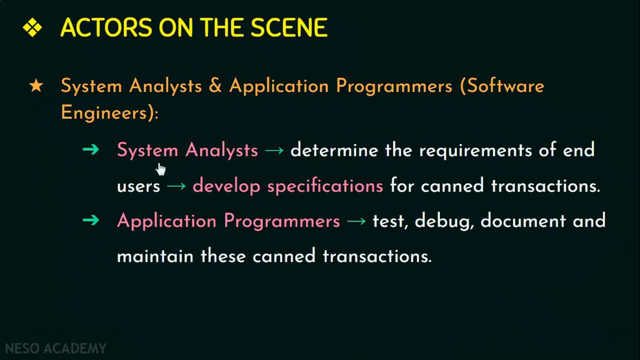 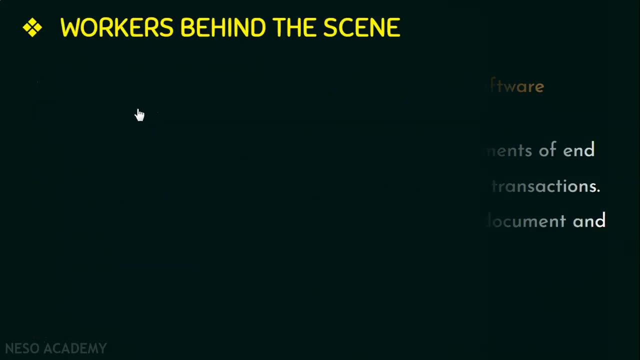 these canned transactions that are developed by the system analysts. These system analysts and application programmers are called as software engineers, And they have to be experts or completely familiar with the facilities provided by the DBMS. Next, let us see the types of database users under the workers behind the scene. 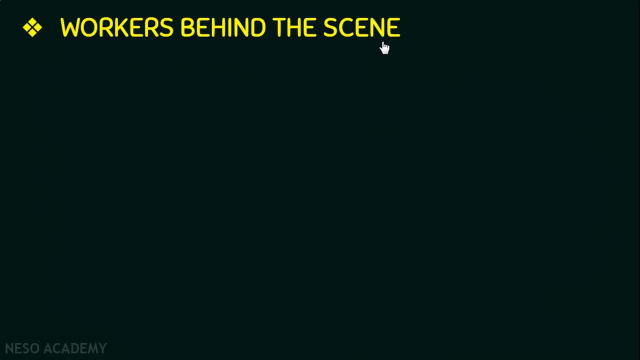 We have already seen, initially, that workers behind the scene are the people whose job is to maintain the database system environment, And these people they are not interested in the database itself. That is, they work behind the scene And the types of database users under them are. the first one is System designers and